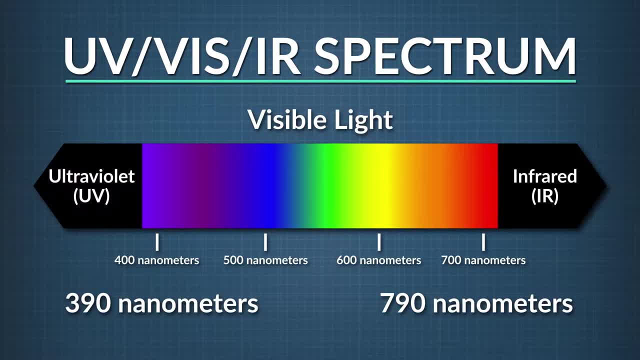 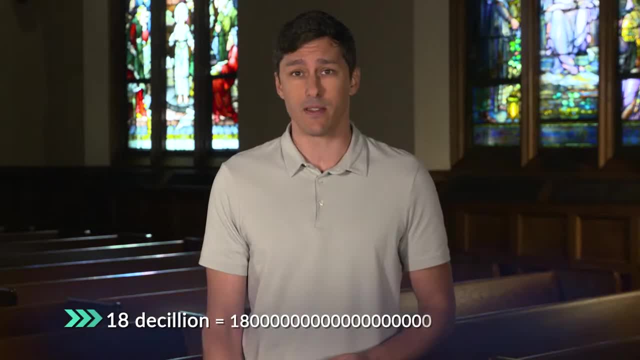 pretty short, One billionth of a meter. How many colors are there in the universe? It's been estimated that we distinguish between 18 decillion colors. That's 18, followed by 33 zeros. A lot of choice, huh. 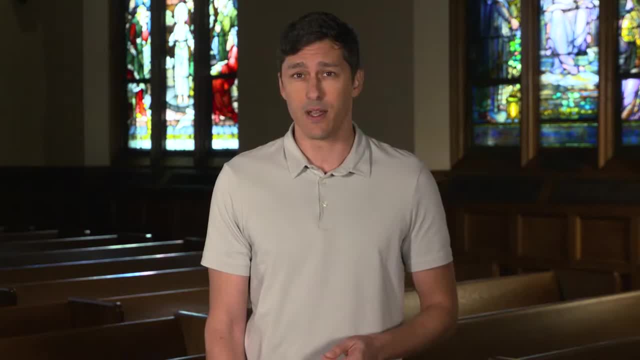 You may have been taught that the three primary colors are red, blue and yellow, But those are the primary colors of pigments, which are substances that add color to materials. The primary colors of light are red, green and blue. Subtitles by the Amaraorg community. 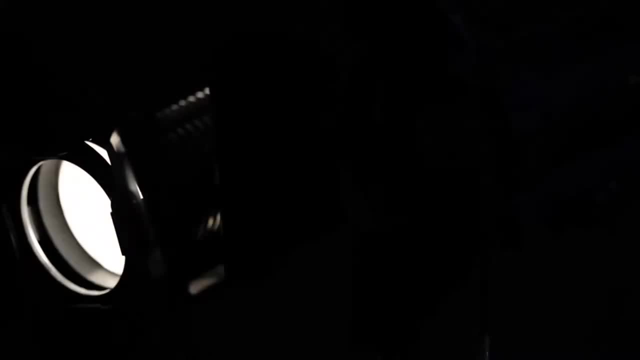 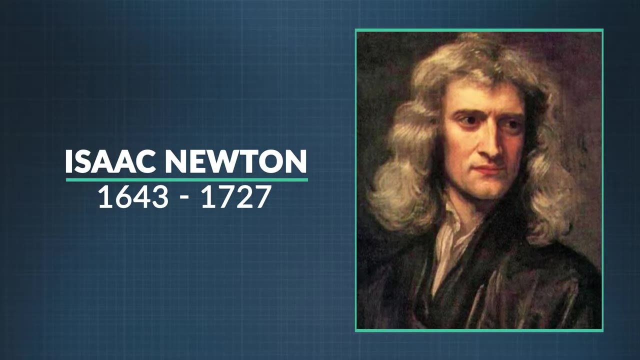 But what happens? when you mix all three of those, We get this White light. It was that genius of physics we've heard a lot about in this series, Isaac Newton, who figured out that combinations of wavelengths spread out along the visible spectrum make 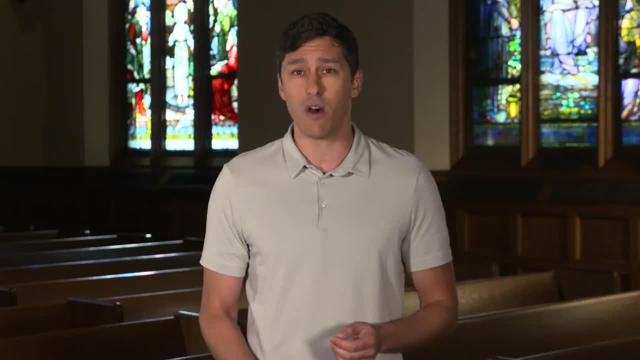 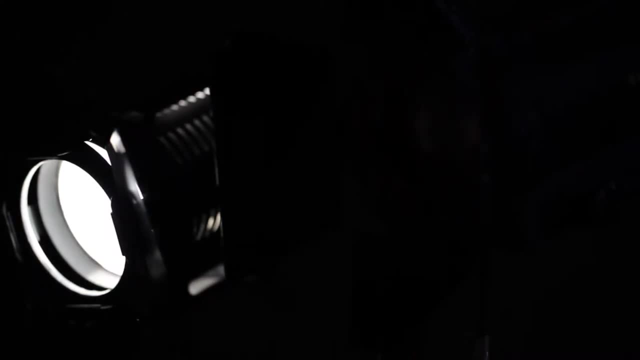 up white light. So white actually isn't a color at all. It is the presence of all of the colors of visible light. He also understood that what we see as black is the absence of light. We see color when white light is the absence of light. 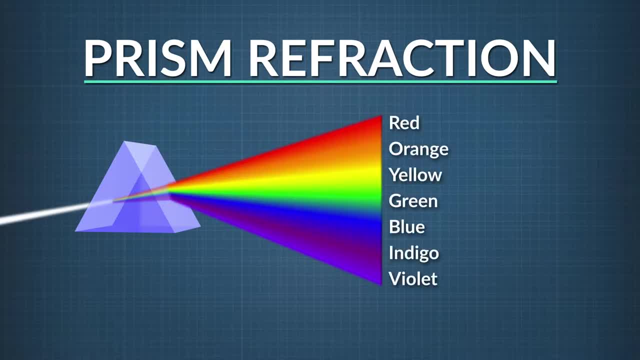 Subtitles by the Amaraorg community. White light is refracted or bent at an angle. The wavelengths are distributed along a spectrum, what we often think of as a rainbow. We'll talk more about color a bit later, but there are other cool characteristics of light and we're in a good spot to talk about those. 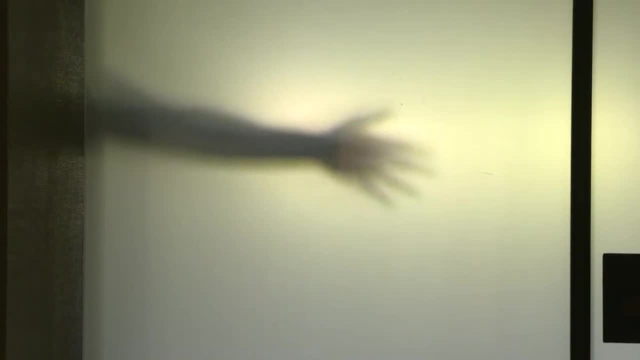 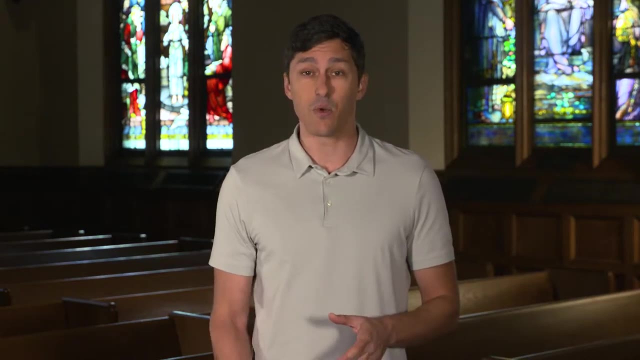 See how the light comes through the window, But the glass is not clear, is it? If the material that light is moving through is rough, even microscopically rough, it will diffuse or spread out the light. Subtitles by the Amaraorg community. 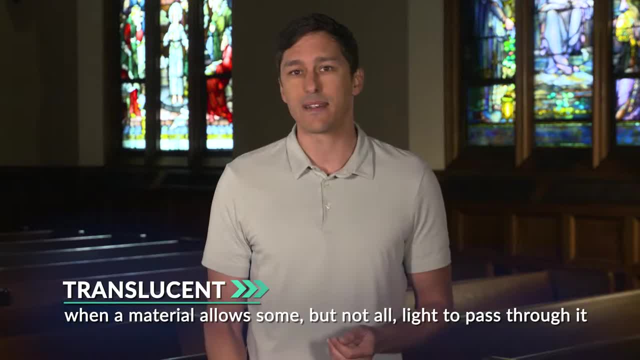 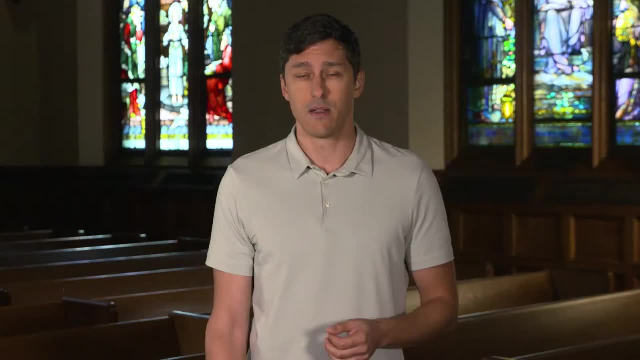 We call that kind of material translucent, and that's what this glass is. It's a medium that allows some, but not all, light to pass through it, so the objects cannot be seen clearly. If no light passes through a material at all, we say that material is opaque. If 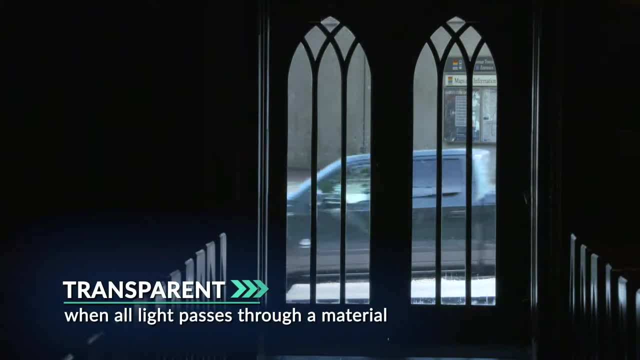 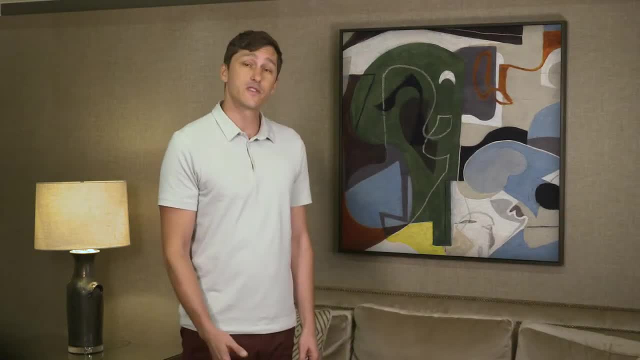 all the light passes through a material, like through this window. the material is transparent. Look at this painting Now. look at it. Looks a lot brighter, doesn't it? That's because the light we just turned on is reflecting off the surface of the painting. We call that. 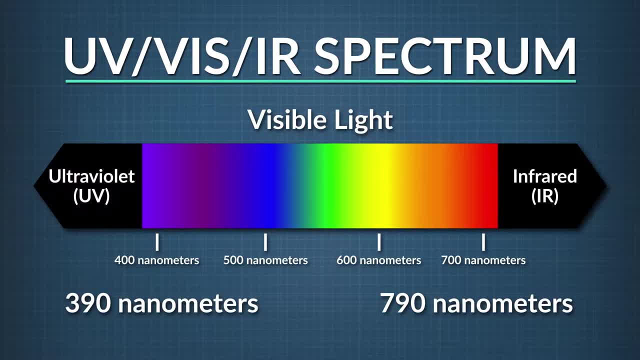 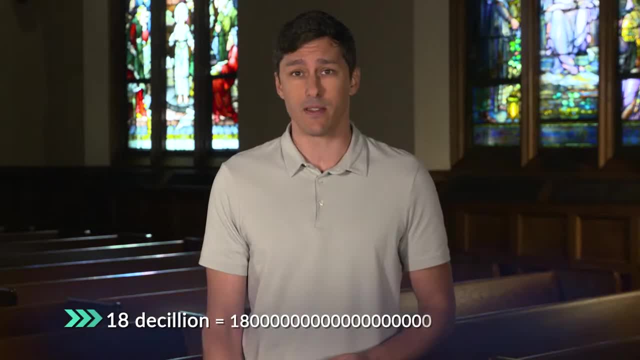 pretty short, One billionth of a meter. How many colors are there in the universe? It's been estimated that we distinguish between 18 decillion colors. That's 18, followed by 33 zeros. A lot of choice, huh. 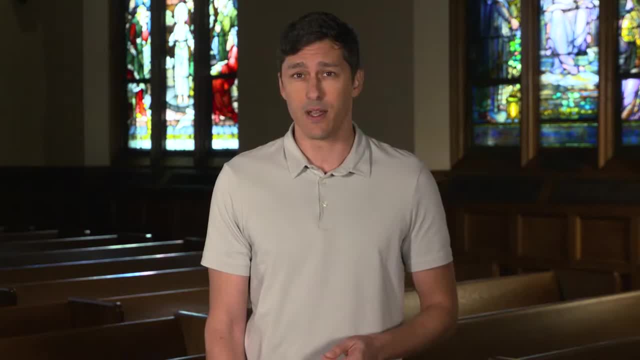 You may have been taught that the three primary colors are red, blue and yellow, But those are the primary colors of pigments, which are substances that add color to materials. The primary colors of light are red, green and blue. Subtitles by the Amaraorg community. 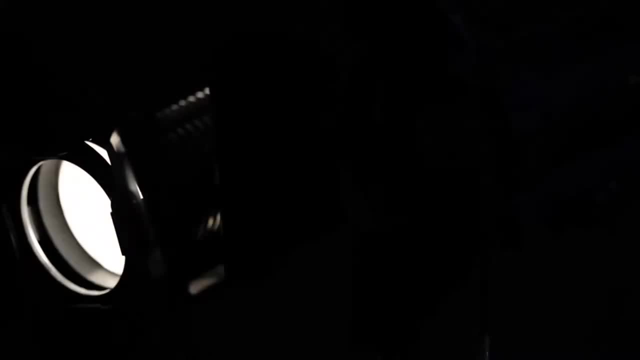 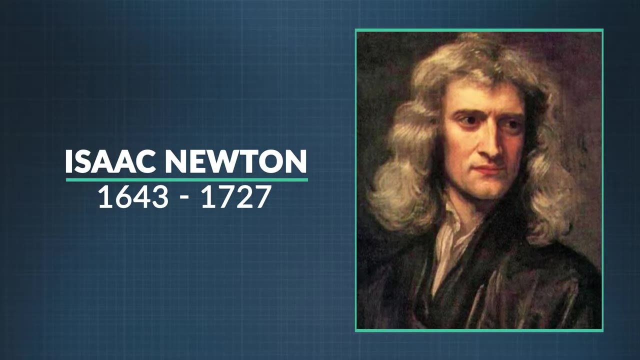 But what happens? when you mix all three of those, We get this White light. It was that genius of physics we've heard a lot about in this series, Isaac Newton, who figured out that combinations of wavelengths spread out along the visible spectrum make 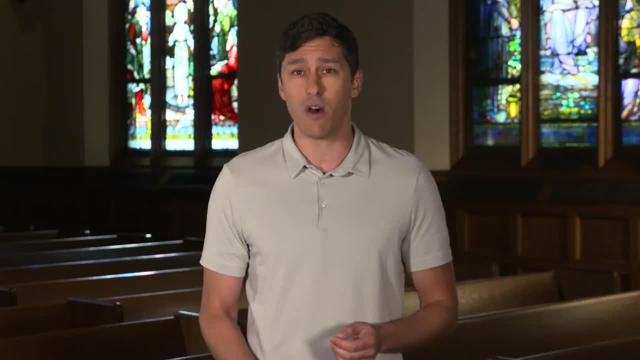 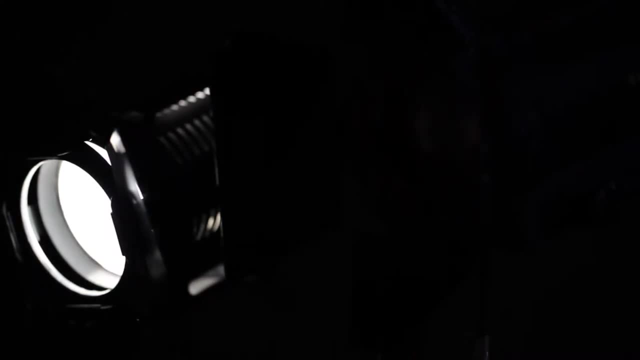 up white light. So white actually isn't a color at all. It is the presence of all of the colors of visible light. He also understood that what we see as black is the absence of light. We see color when white light is the absence of light. 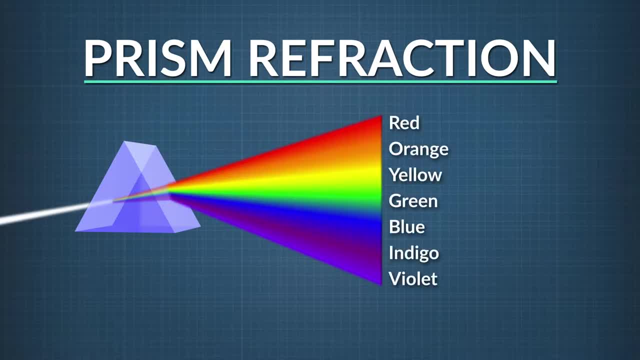 Subtitles by the Amaraorg community. White light is refracted or bent at an angle. The wavelengths are distributed along a spectrum, what we often think of as a rainbow. We'll talk more about color a bit later, but there are other cool characteristics of light and we're in a good spot to talk about those. 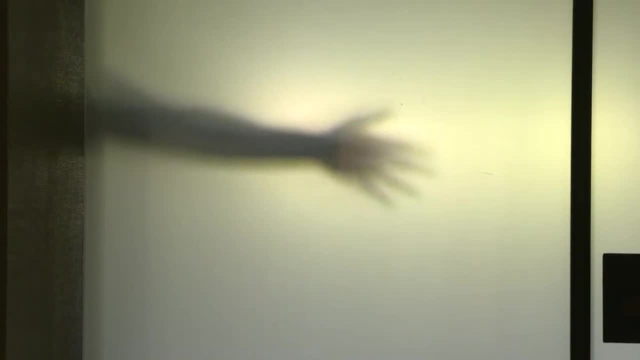 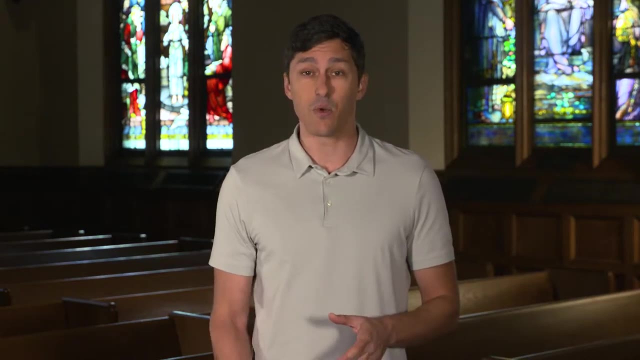 See how the light comes through the window, But the glass is not clear, is it? If the material that light is moving through is rough, even microscopically rough, it will diffuse or spread out the light. Subtitles by the Amaraorg community. 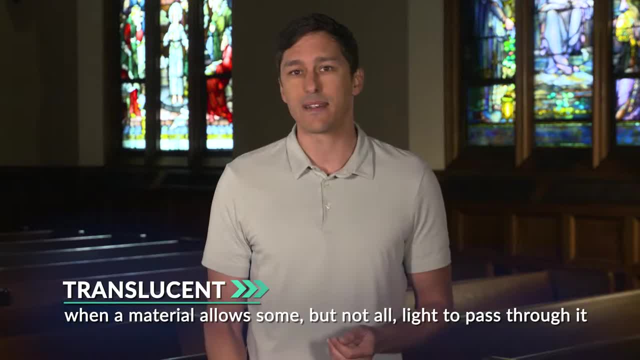 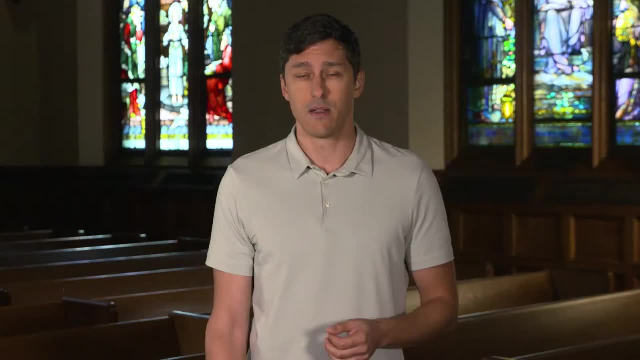 We call that kind of material translucent, and that's what this glass is. It's a medium that allows some, but not all, light to pass through it, so the objects cannot be seen clearly. If no light passes through a material at all, we say that material is opaque. If 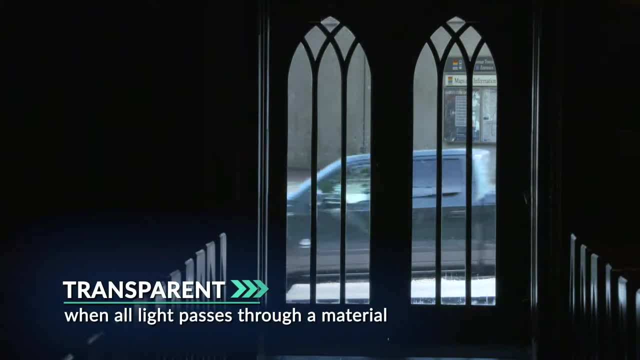 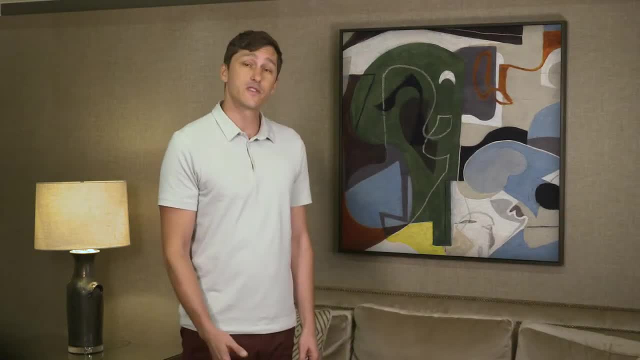 all the light passes through a material, like through this window. the material is transparent. Look at this painting Now. look at it. Looks a lot brighter, doesn't it? That's because the light we just turned on is reflecting off the surface of the painting. We call that. 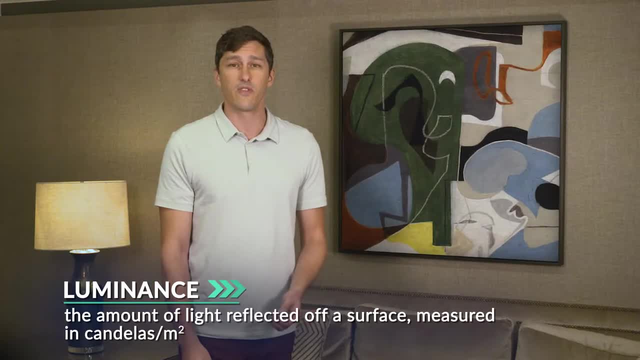 measure of brightness: luminance, which is the amount of light reflected off a surface measured in candelas per square meter. The unit you might be more familiar with, lumens, is the unit for luminous intensity, which measures the brightness of light in a given. 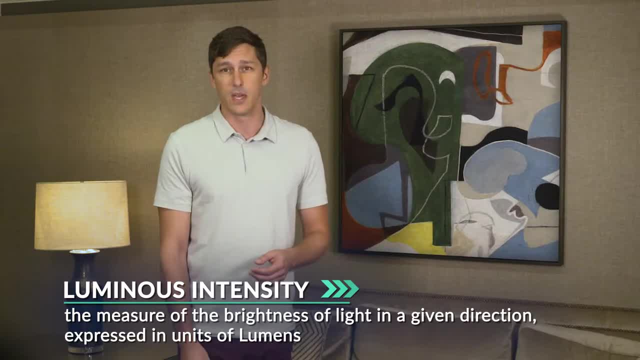 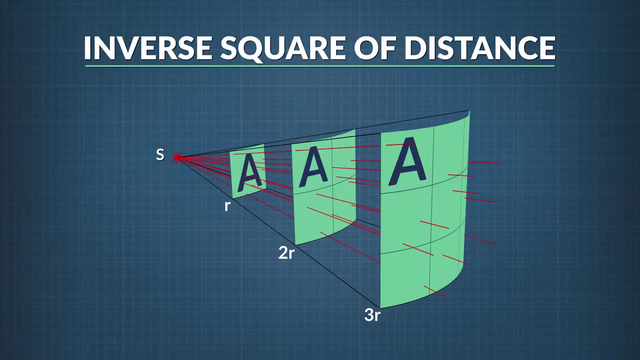 direction. You can see that word on any light bulb package. It's different than wattage, which measures the electrical power a device uses. This is inversely related to the square of the distance from the light source. The farther away you are, the less the luminance, The brightness, decreases at an exponential rate. 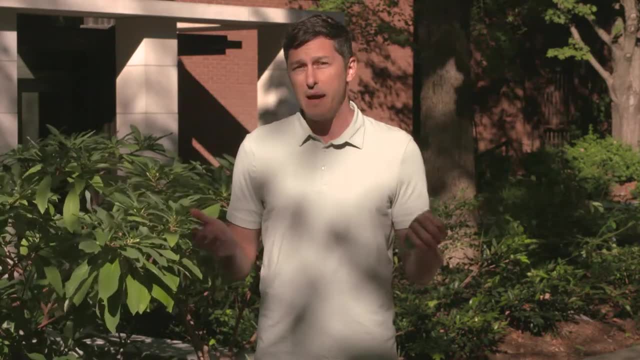 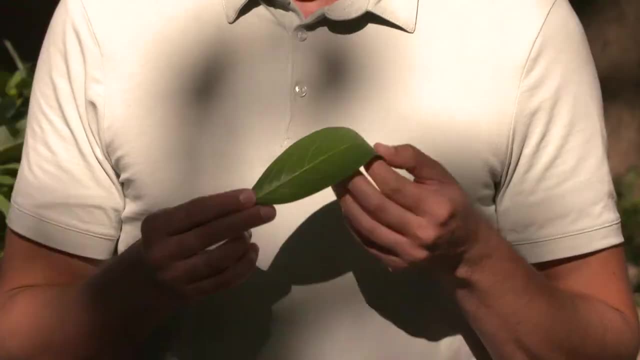 Now that we've talked about some characteristics of the way light behaves, we've come outside to show you something awesome that goes on every day all over the planet: All this green. But why does this leaf look green? Because it's reflecting the wavelength of green light. 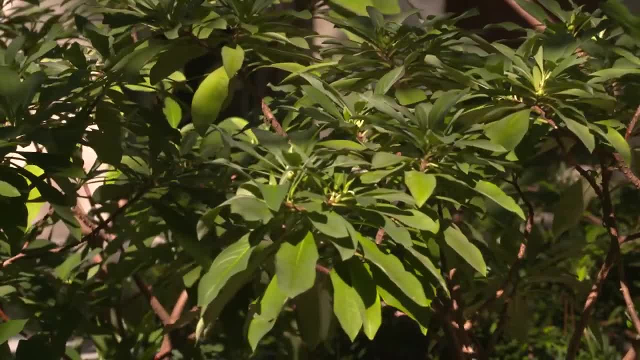 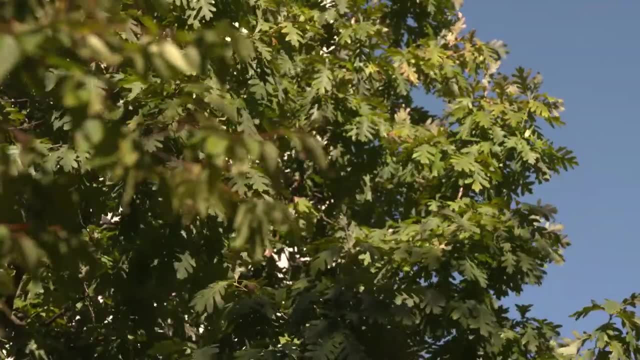 and absorbing all the other colors. The chemical that makes this happen is chlorophyll, which, you might know, is involved in photosynthesis, the process that plants use to make nutrients out of light. Chlorophyll is a light-trapping pigment. It absorbs red light, which is the most effective wavelength when it comes to 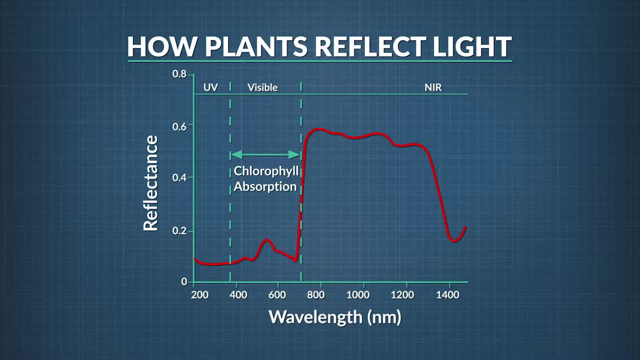 making glucose, a form of sugar, from light. What we call the red edge, near the infrared end of the spectrum, is where photosynthesis for plants is most active. So we have our own little factory going on here, powered by absorbed light, near the infrared part of 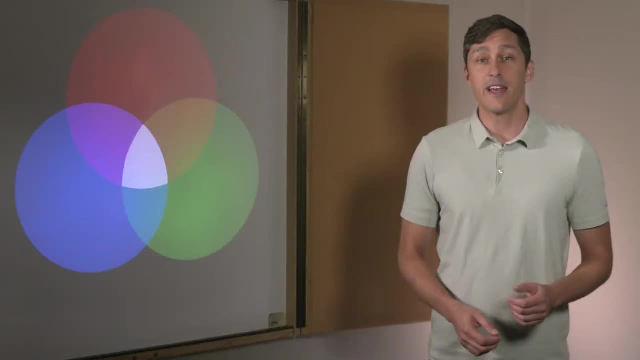 the spectrum. Let's explore more about color in our everyday world. We brought in this color projector to do just that. Remember, our primary colors of light are red, green and blue. They are specific wavelengths of light. When we overlap all three of them in equal intensities, we 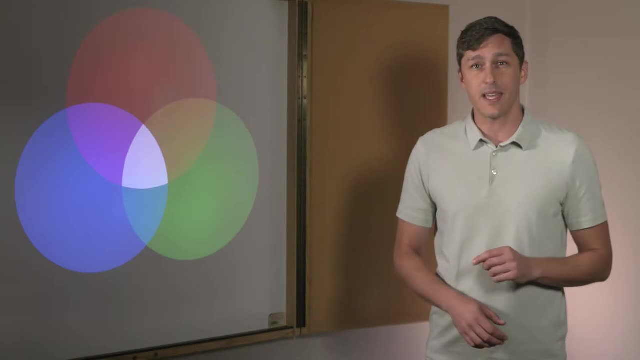 get white light. Where the three primary colors come together, you can see a small triangle of white light. Why? What do you remember about the nature of color? Let's go inside and take a look. When we overlap two of the primary colors, we get. 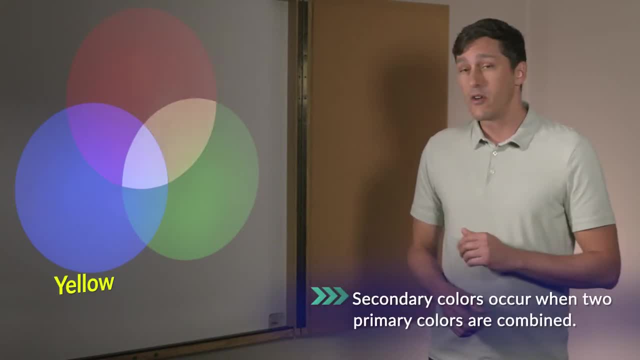 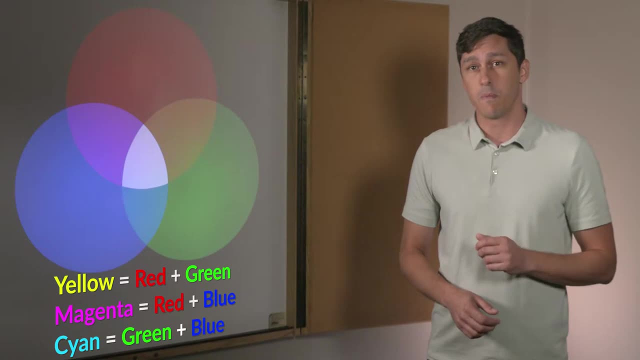 what we call the secondary colors of light, which are yellow from combining red and green, magenta from combining red and blue, and cyan from combining green and blue. That may sound familiar from your printers' ink cartridges. We'll talk about that more. 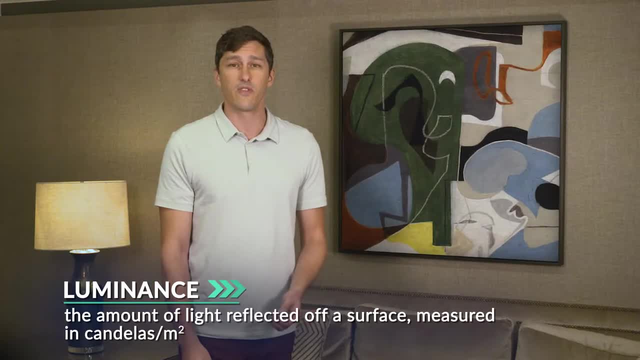 measure of brightness: luminance, which is the amount of light reflected off a surface measured in candelas per square meter. The unit you might be more familiar with, lumens, is the unit for luminous intensity, which measures the brightness of light in a given. 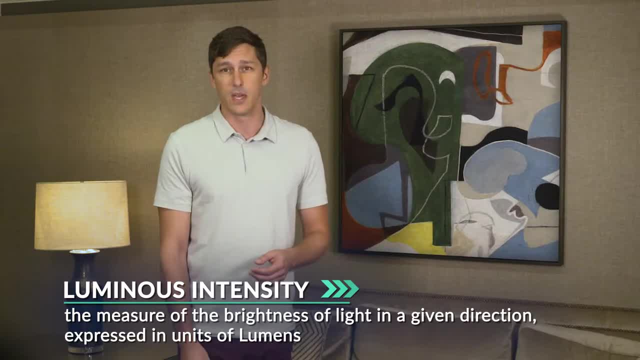 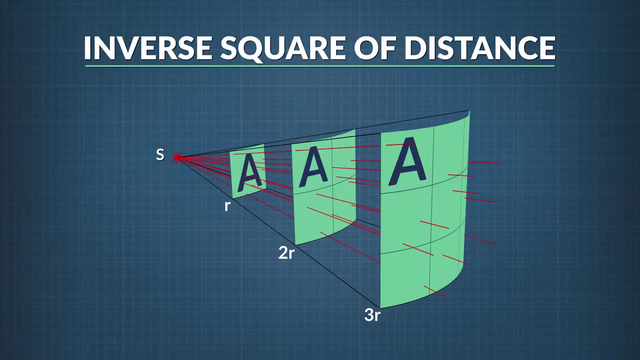 direction. You can see that word on any light bulb package. It's different than wattage, which measures the electrical power a device uses. This is inversely related to the square of the distance from the light source. The farther away you are, the less the luminance, The brightness, decreases at an exponential rate. 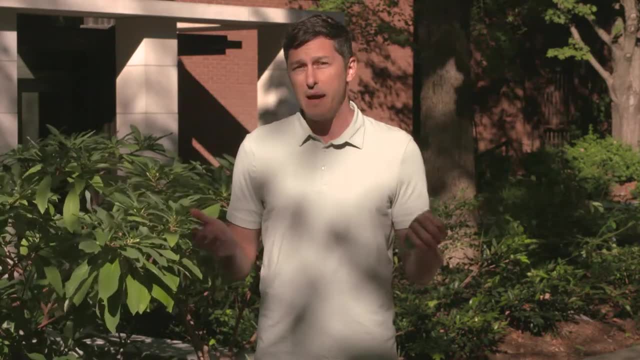 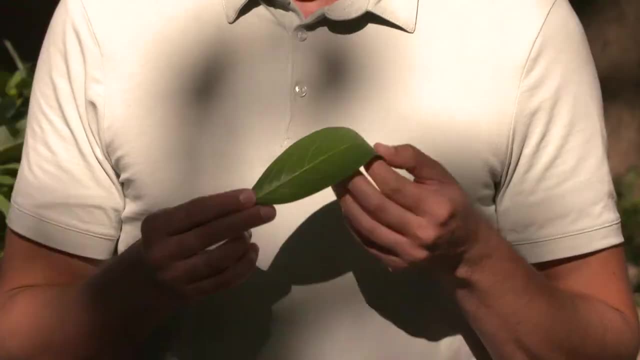 Now that we've talked about some characteristics of the way light behaves, we've come outside to show you something awesome that goes on every day all over the planet: All this green. But why does this leaf look green? Because it's reflecting the wavelength of green light. 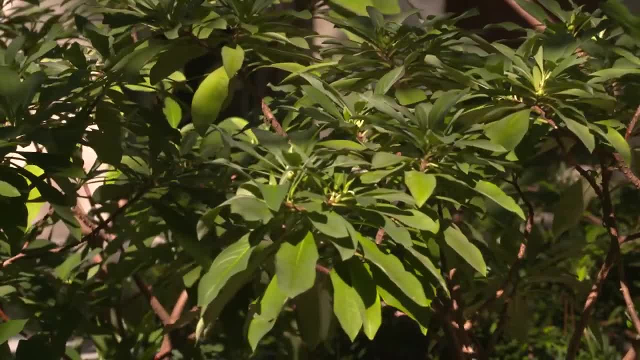 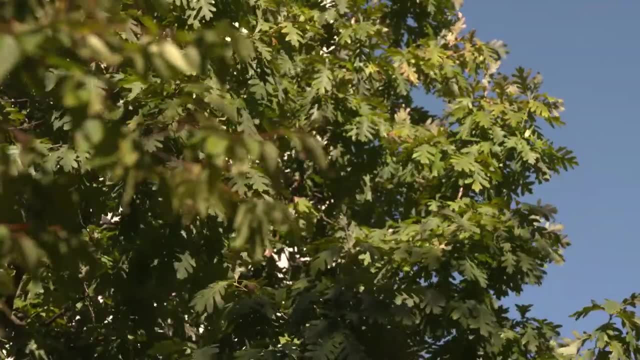 and absorbing all the other colors. The chemical that makes this happen is chlorophyll, which, you might know, is involved in photosynthesis, the process that plants use to make nutrients out of light. Chlorophyll is a light-trapping pigment. It absorbs red light, which is the most effective wavelength when it comes to 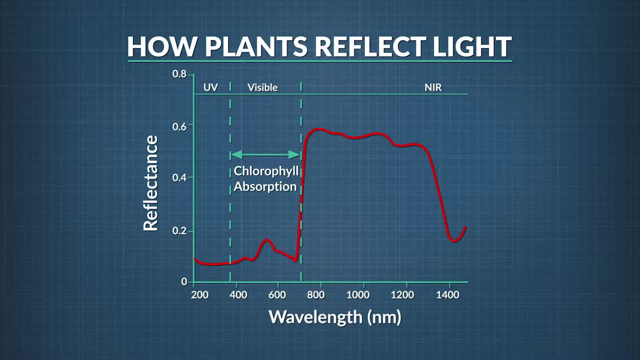 making glucose, a form of sugar, from light. What we call the red edge, near the infrared end of the spectrum, is where photosynthesis for plants is most active. So we have our own little factory going on here, powered by absorbed light, near the infrared part of 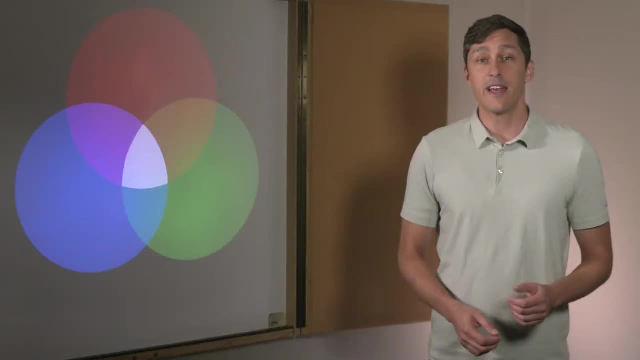 the spectrum. Let's explore more about color in our everyday world. We brought in this color projector to do just that. Remember, our primary colors of light are red, green and blue. They are specific wavelengths of light. When we overlap all three of them in equal intensities, we 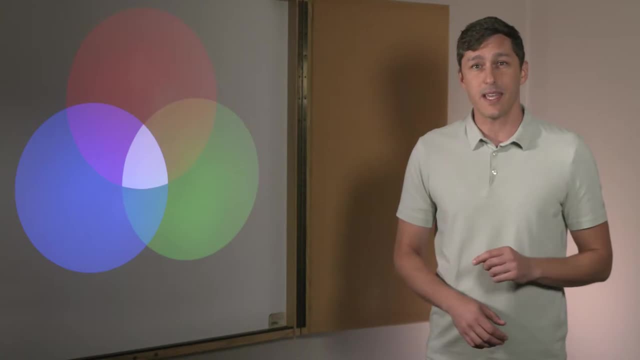 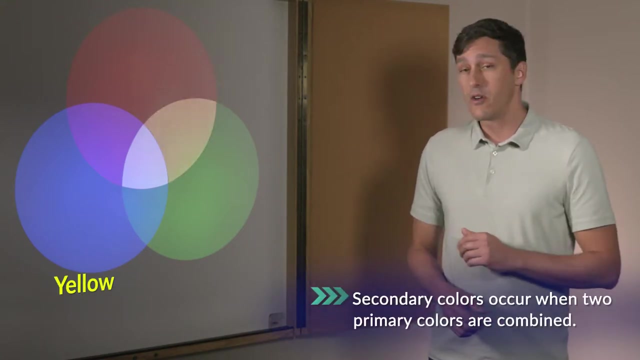 get white light. Where the three primary colors come together, you can see a small triangle of white light. Why? What do you remember about the nature of color? When we overlap two of the primary colors, we get what we call the secondary colors of light, which are yellow. 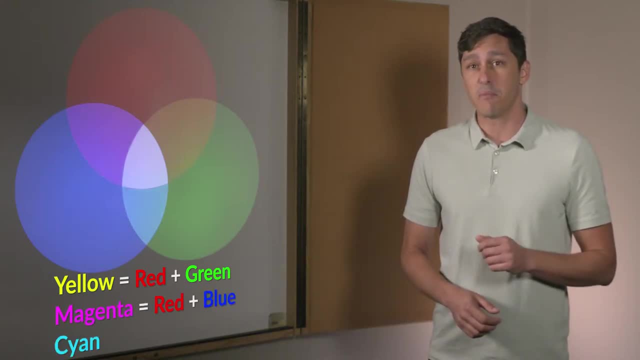 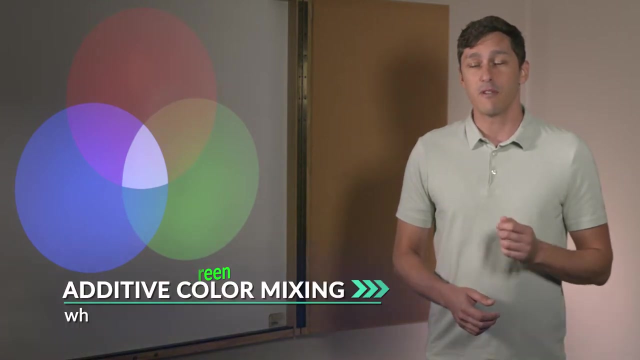 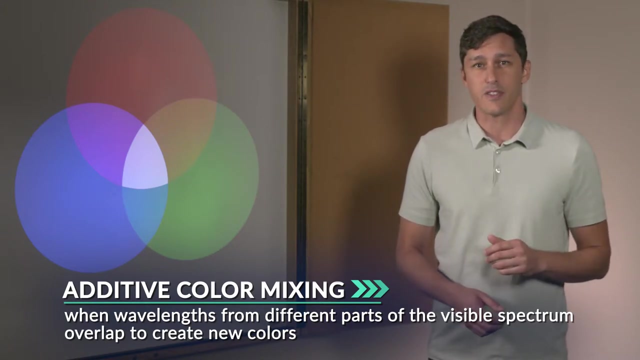 magenta and cyan. That may sound familiar from your printer's ink cartridges. But what about the amazing array of colors we can see from light? They arise from what we call additive color mixing, when wavelengths from different parts of the visible spectrum overlap to create subtle, beautiful and endless colors. 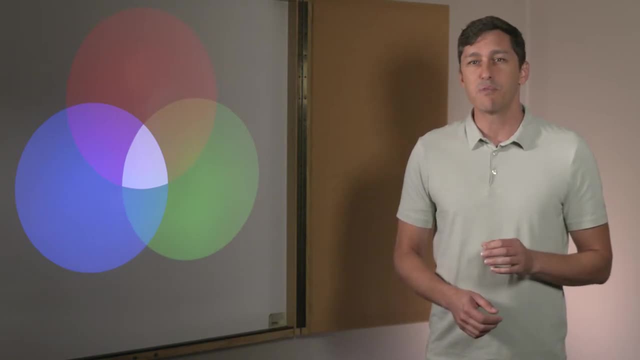 By blending different wavelengths of light from the visible spectrum, I can produce any color of light I want. Within additive color mixing, we can also produce white light using complementary colors. These are pairs of colors which, when combined, produce white light. For example, some complementary combination of colors are green and magenta, blue and. 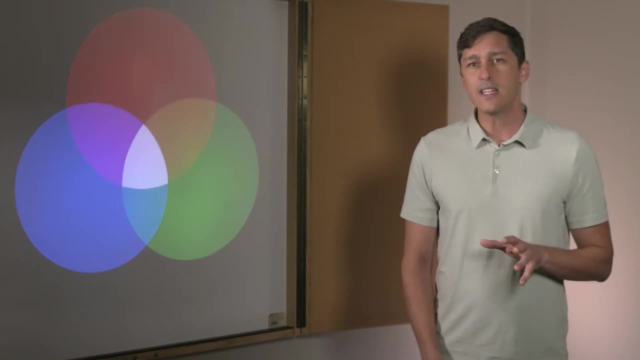 yellow, red and cyan. When any two of them are combined, they do a very specific thing. Let's look at green and magenta now yellow and blue and red and cyan- See all produce white light. Each of these pairs is made of one primary color and a secondary color. 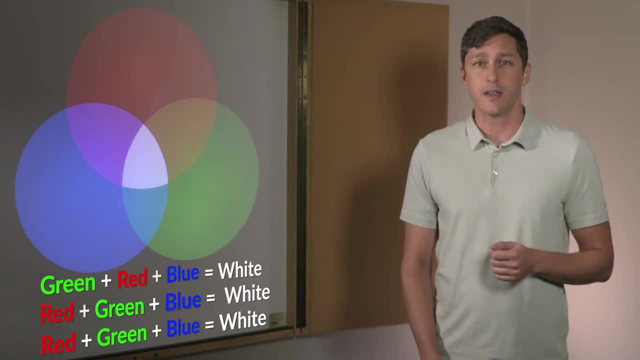 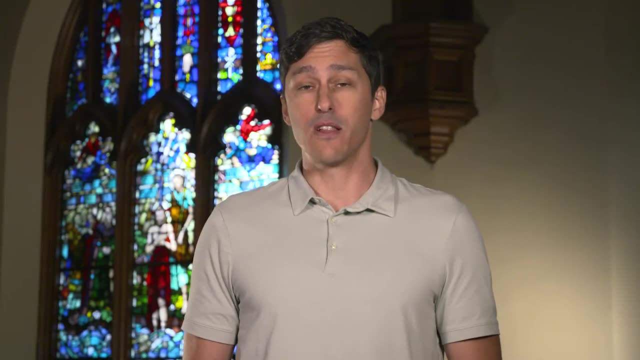 The secondary colors themselves are made of two other primary colors, allowing for all of the wavelengths of light to be present to create white light. There's another kind of color mixing by light. It's called subtractive. This is when materials reflect and absorb light rather than only reflecting it as 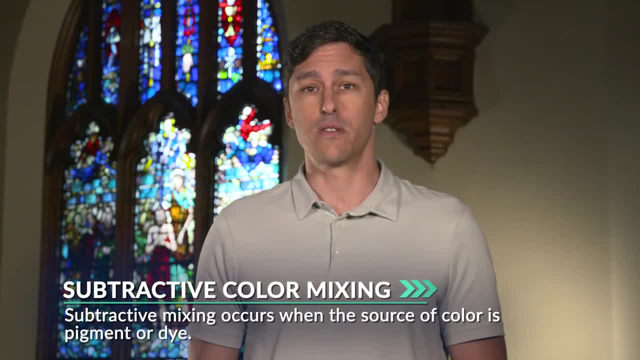 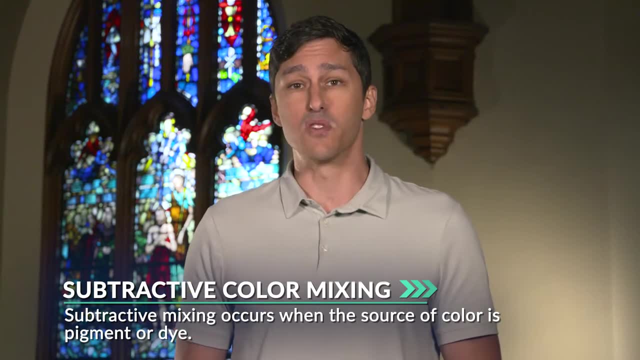 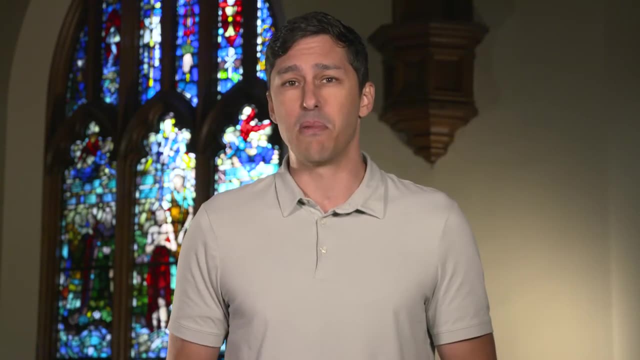 in additive color mixing. Subtractive mixing occurs when the source of color is pigment or dye. The refractive properties of the molecules within the pigments and dyes absorb some wavelengths of light and reflect others. So when these dyes subtract or take away the wavelengths by absorbing them, we are 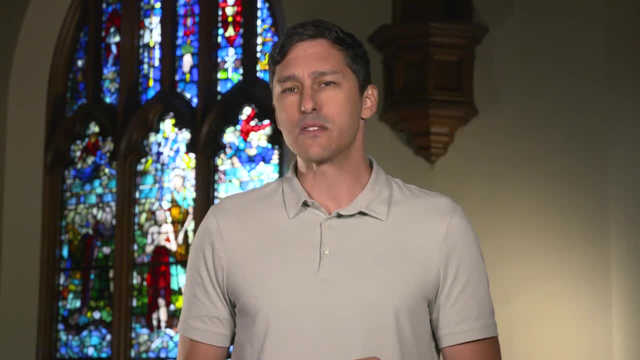 left with the colors that are reflected. Subtractive mixing: If you mix too many pigments so that all the wavelengths are being absorbed, what would you get? Almost black, because nothing is being reflected. Mixing paints is the exact opposite of mixing light, and here's an example of how painters 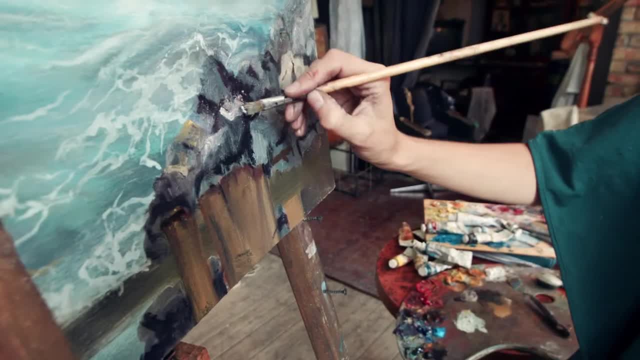 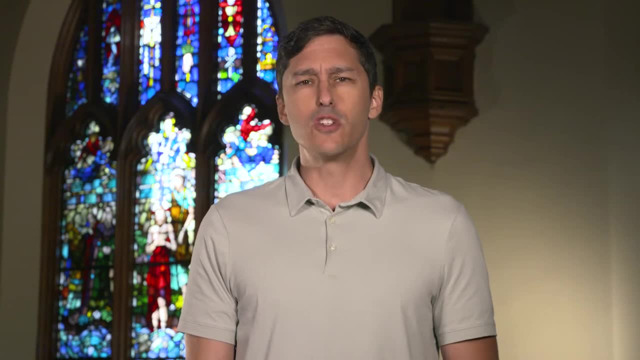 use their properties to create an amazing array of colors. We can add color to objects like materials or canvas in a few ways. Pigment is one which is usually made from inorganic sources that change the color of reflected or transmitted light. Subtractive mixing: 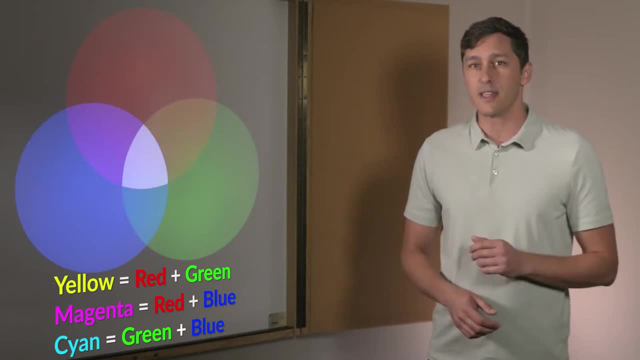 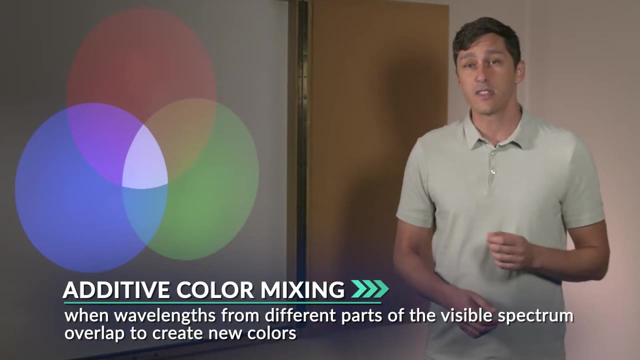 in a moment. But what about the amazing array of colors we can see from light? They arise from what we call additive color mixing, When wavelengths from different parts of the visible spectrum overlap to create subtle, beautiful and endless colors By blending different. 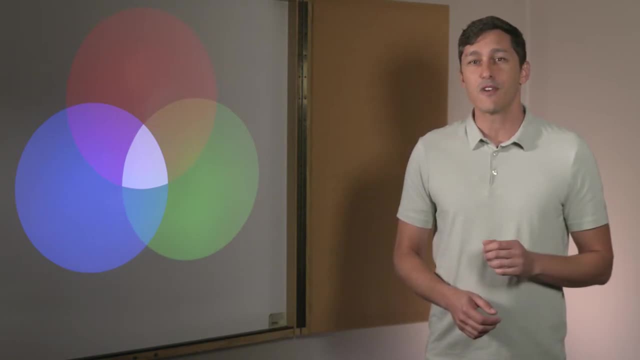 wavelengths of light from the visible spectrum, I can produce any color of light I want Within additive color mixing. we can also produce white light using complementary colors. These are pairs of colors which, when combined, produce white light. For example, some complementary: 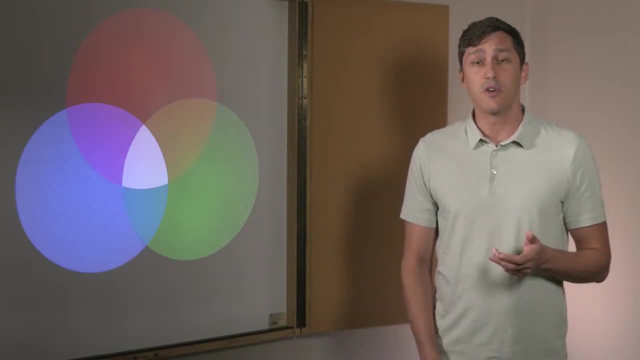 combination of colors are green and magenta, blue and yellow, red and cyan. When any two of them are combined, they do a very specific thing. Let's look at green and magenta now, yellow and blue and red and cyan See all produce white light. Each of these pairs is 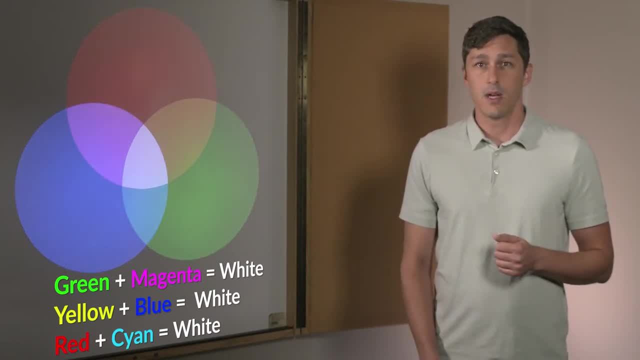 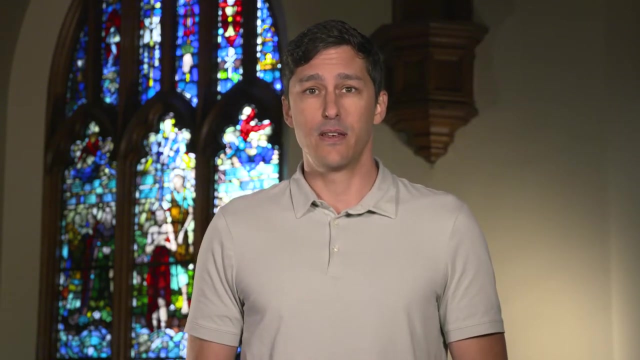 made of one primary color and a secondary color. The secondary colors themselves are made of two other primary colors, allowing for all of the wavelengths of light to be present to create white light. There's another kind of color mixing by light. It's called subtractive. This is when materials reflect and absorb light rather than only. 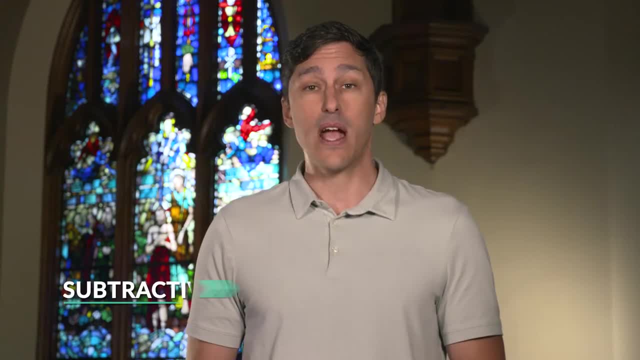 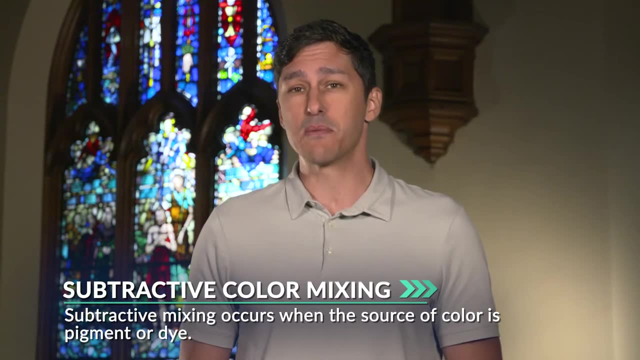 reflecting it, as in additive color mixing. Subtractive mixing occurs when the source of color is pigment or dye. The refractive properties of the molecules within the pigments and dyes absorb some wavelengths of light and reflect others. So when these dyes subtract, 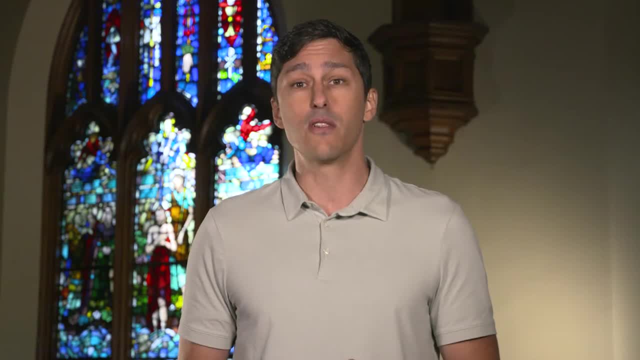 or take away the wavelengths. by absorbing them, we are left with the colors that are reflected. If you mix too many different colors at the same time, the colors will not be reflected in the pigments. If you mix too many pigments so that all the wavelengths are being absorbed, what would 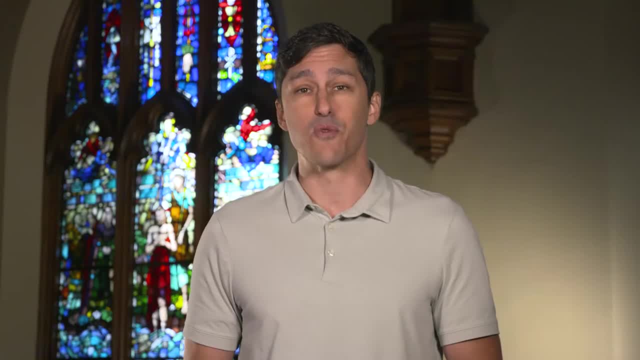 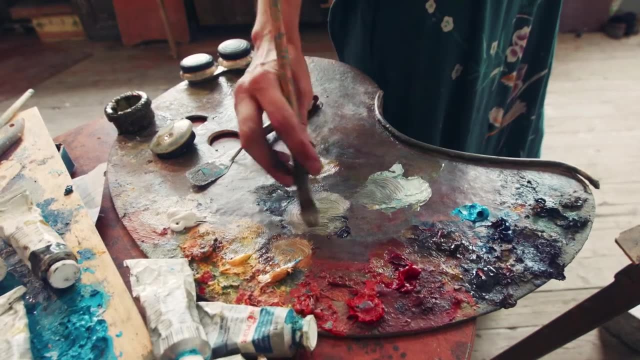 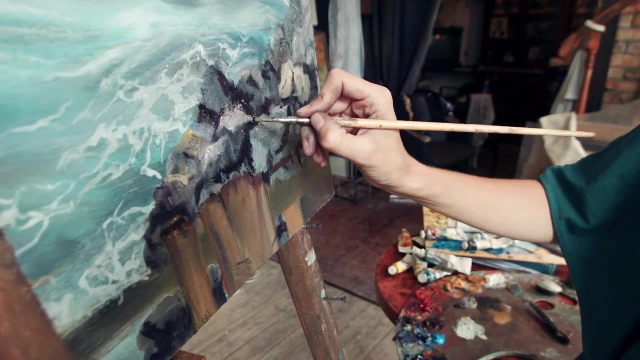 you get Almost black because nothing is being reflected. Mixing paints is the exact opposite of mixing light, and here's an example of how painters use their properties to create an amazing array of colors. We can add color to objects like materials or canvas in a few ways. Pigment is one which